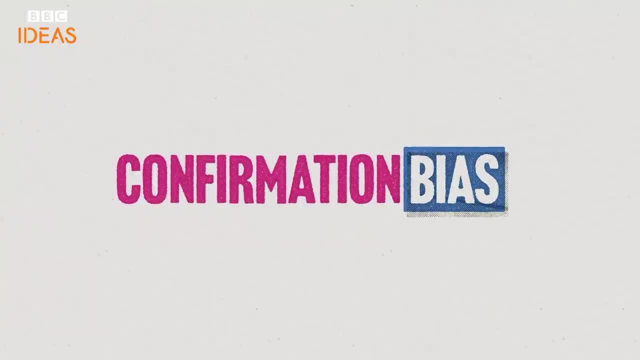 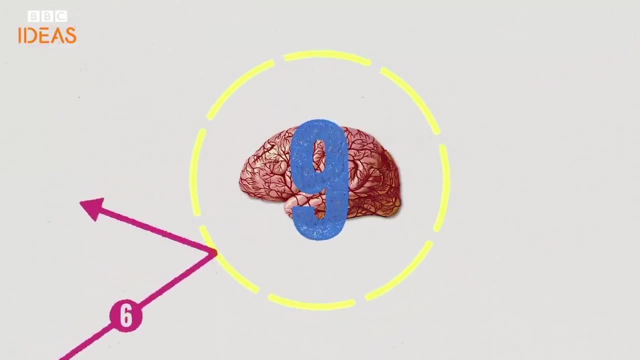 if it contradicts our views. It's what's known as confirmation bias. It's one of the key cognitive biases that humans have and it operates at an unconscious level, affecting our ability to process information. This is especially true for issues which are emotionally. 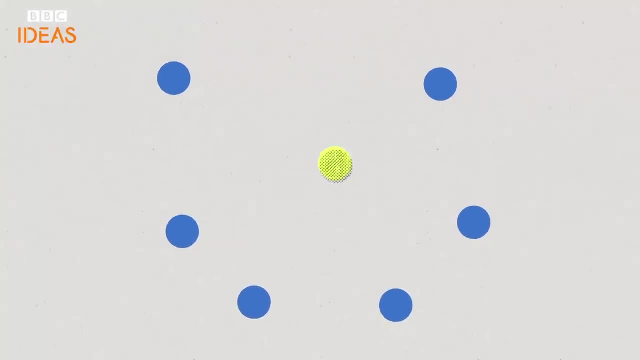 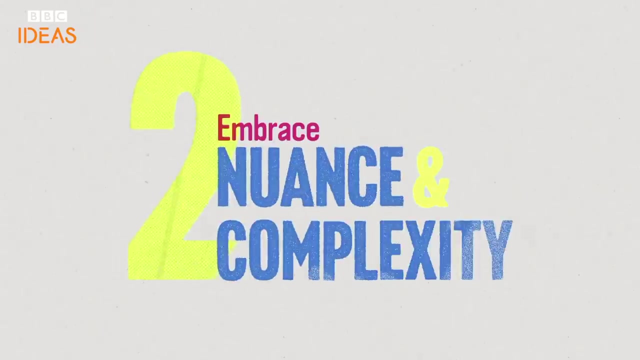 charged or where our views are deeply held. but it can come into play at any time, So don't worry about it, It's just a matter of time. Don't rush to decide and be actively prepared to change your mind. So many of our discussions take place on social media platforms, where algorithms reward our 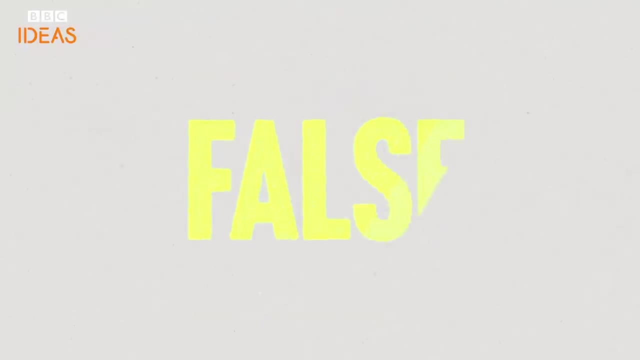 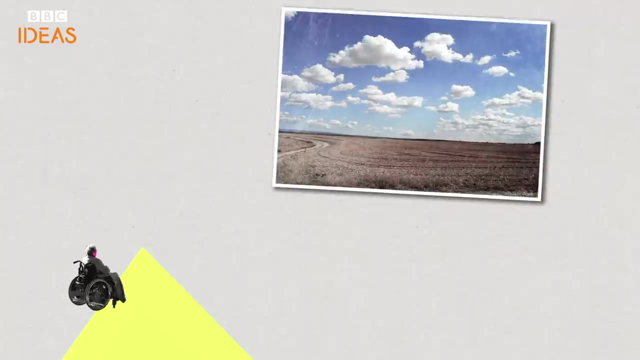 desire to see and hear our views confirmed, But in life, most situations are nuanced and complicated. Acknowledging that can enrich the way that we view the world. For example, what colour is the sky? Well, the obvious answer is blue, But at sunrise or sunset. 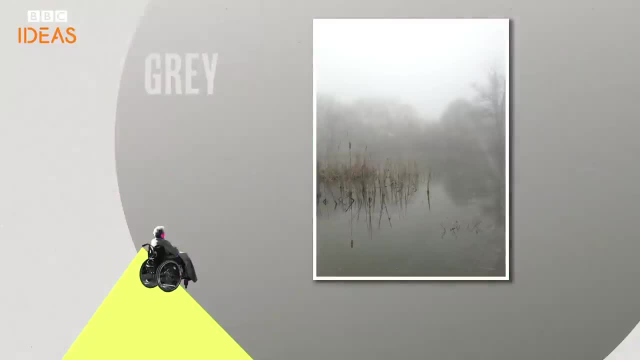 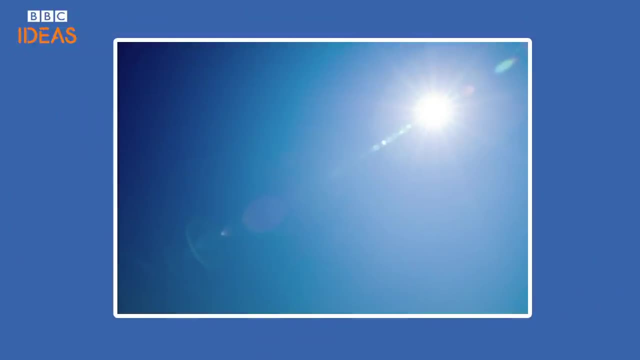 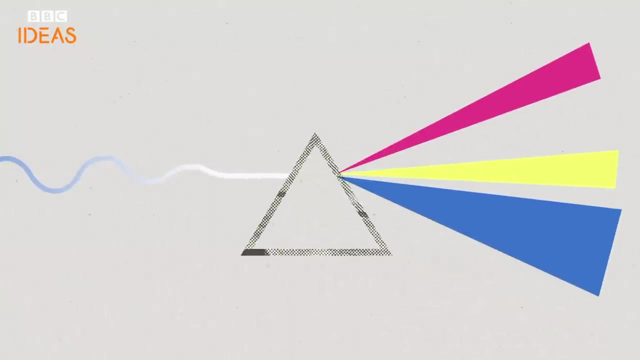 it can be red On a cold, misty morning, white or grey At night, midnight blue or black. But imagine for a moment the blue of the sky on a sunny day. Is it really blue? The colour blue has a short wavelength, meaning it scatters more than other colours, making it more visible. 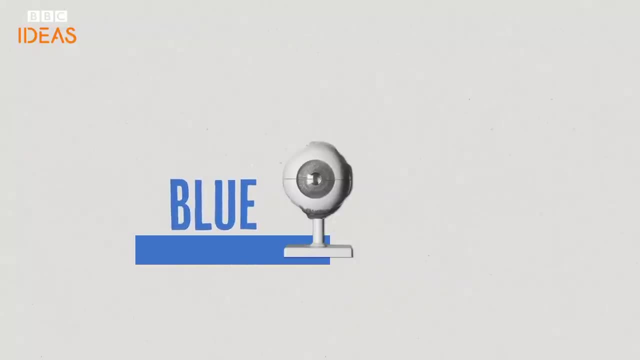 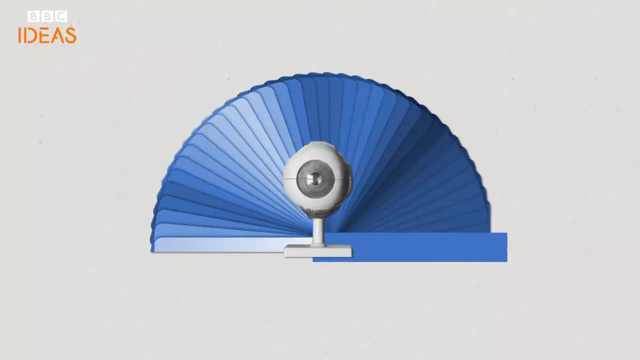 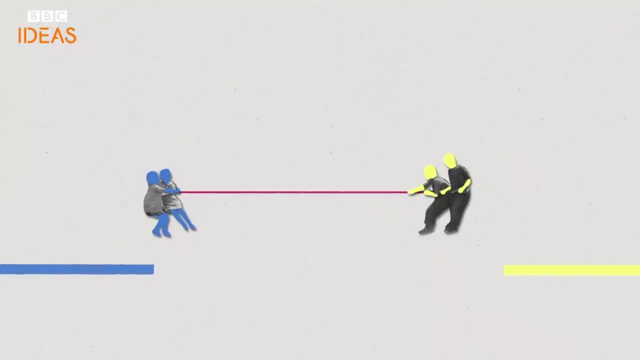 to the human eye. So the sky looks blue to us humans, even though there's a whole spectrum of colours out there. Even something that seems totally self-evident can be more nuanced than you think. One approach to well arguing is to let go of the idea of being right, Or at least seriously. 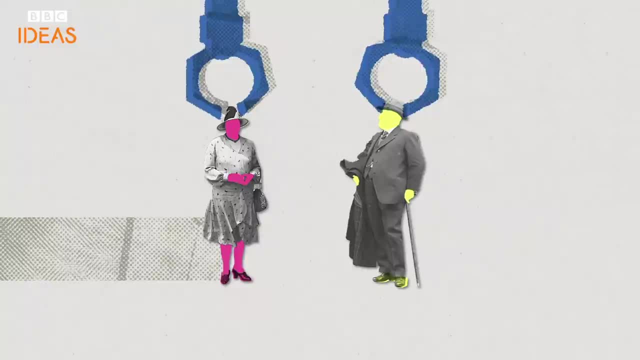 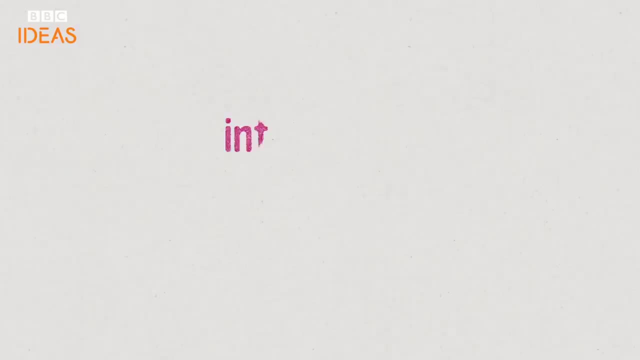 consider that you might actually be wrong. Putting yourself in the other person's shoes can lead to much more productive outcomes. Really try to understand where the other person is coming from. It's what's called intellectual empathy. It can be challenging, but that's.